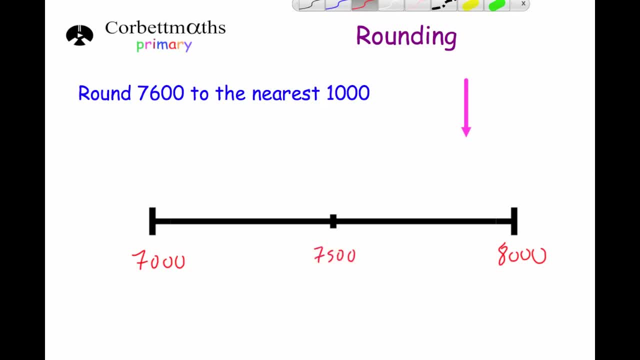 midway between those two numbers would be 7,500.. So that means that 7,600 would be round about here somewhere because it's bigger than 7,500. So that means that 7,600 is closer to 8,000 than it is to. 7,000.. So our answer would be: 7,600 is closer to 8,000 than it is to 7,500.. So that means that 7,600 is closer to 8,000 than it is to 7,500. So that means that 7,600 is closer to 8,000 than it is to. 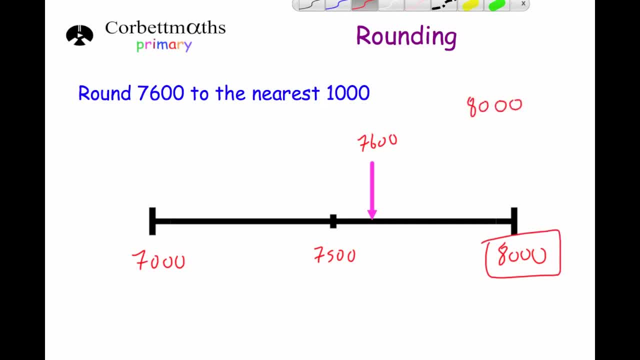 8,000.. Okay, our next question. Our next question asks us to round 8,531 to the nearest thousand. So again, the multiples of thousand close to 8,531 would be 8,000 and 9,000 and midway between those would. 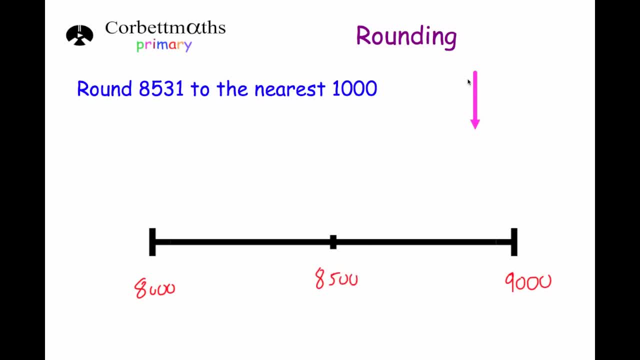 be 8,500.. So if we were asked to put this number on the number line 8,531, well it's going to be here because it's slightly bigger than 8,500.. so that means that our um, that means that eight thousand five hundred and thirty one is closer. 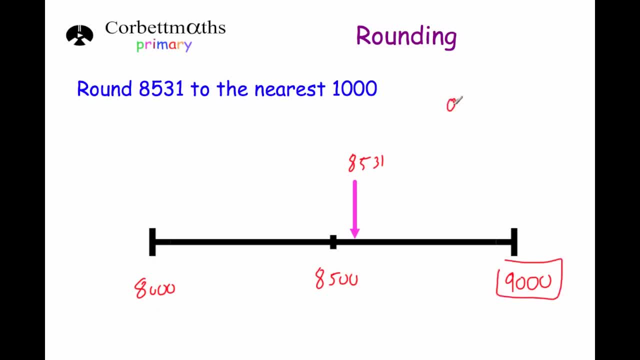 to nine thousand than it is to eight thousand. so our answer would be nine thousand. okay, our next question? our next question asks us to round thirteen thousand four hundred and eighty to the nearest thousand. so thirteen thousand would be the multiple of a thousand, just below that number. 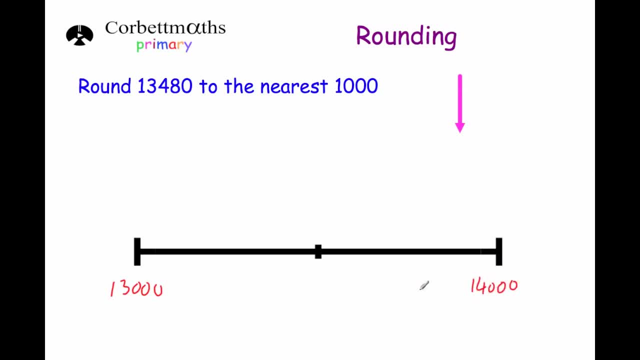 and the multiple thousand just above, it would be fourteen thousand, and in the middle of those two numbers would be thirteen thousand five hundred. now, if we were asked to put this number, thirteen thousand four hundred and eighty- on this number line, it would be round about here somewhere it. 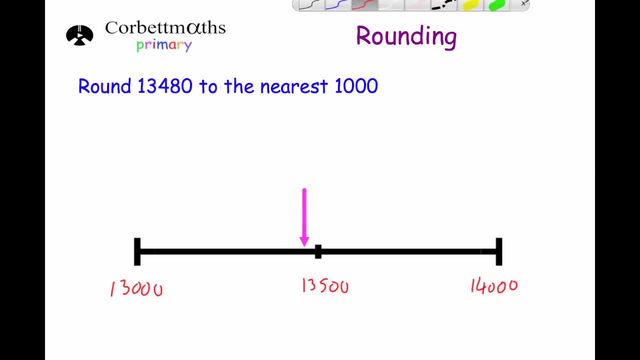 would be just below the thirteen thousand five hundred. so that means that thirteen thousand four hundred and eighty is closer to thirteen thousand than it is to fourteen thousand. so our answer is thirteen thousand. okay, our next question. our next question asks us to round twenty four thousand six hundred and ninety two to the nearest thousand. so 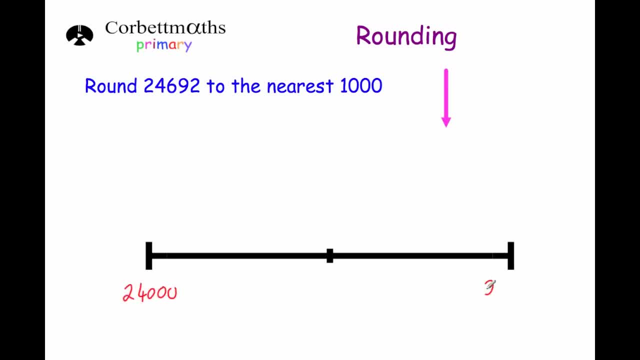 twenty four thousand six hundred and ninety two to the nearest thousand. so twenty four thousand would be the multiple thousand below it and twenty five thousand would be the multiple of a thousand just above it and in the middle would be twenty four thousand five hundred. so if we were asked to, 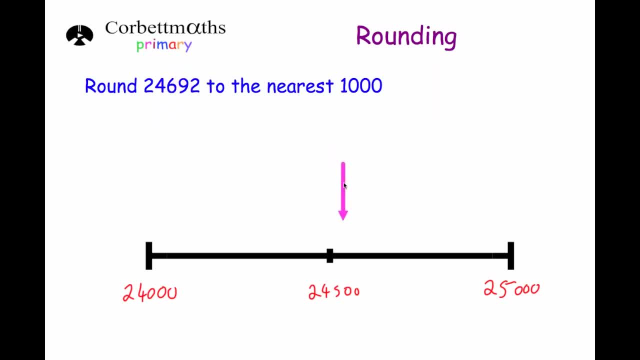 put this number twenty four thousand six hundred and ninety two on the number line, it would be over here somewhere because it's bigger than twenty four thousand five hundred. so that means that twenty four thousand six hundred and ninety two is closer to twenty five thousand than it is.